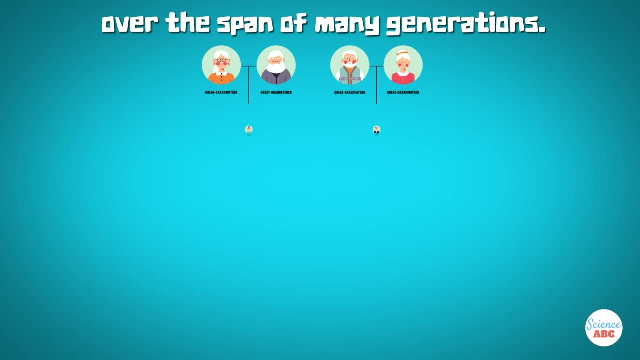 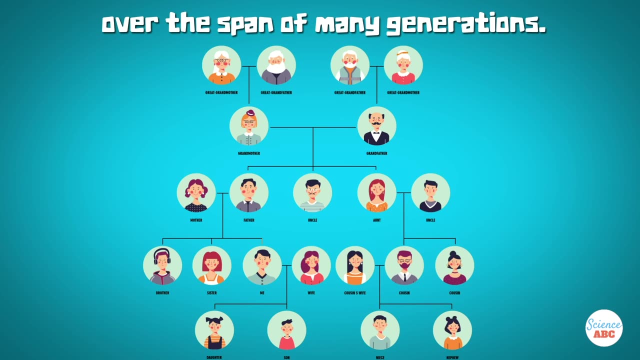 like natural selection. The second part tells us two things: the time it takes for organisms to change and, less obviously, that the process involves reproduction, DNA heritability and change. The core of evolution is the change in organisms. 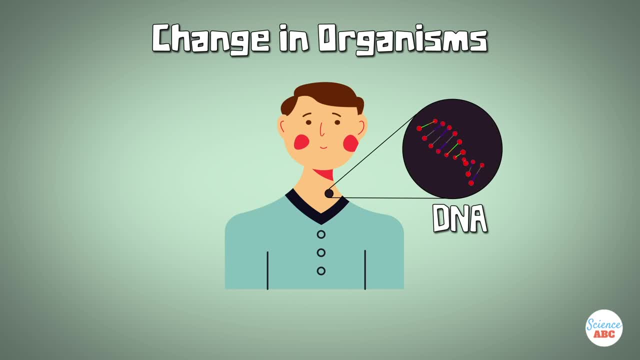 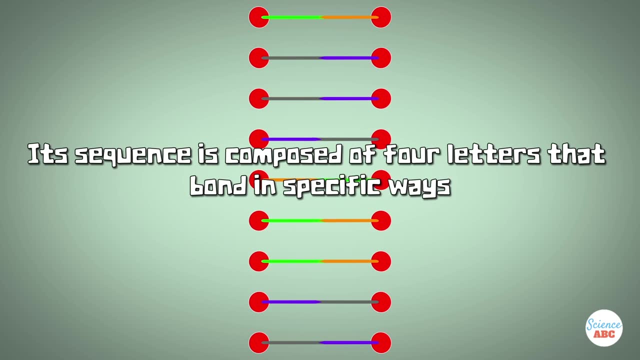 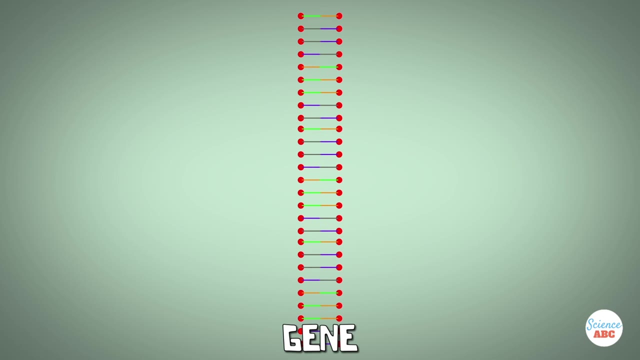 and the first place to investigate this change is the DNA. DNA is the blueprint of all life. Its sequence is composed of four letters that bond in specific ways: A to T and C to G, Small sections of the DNA sequence called genes code for certain traits. 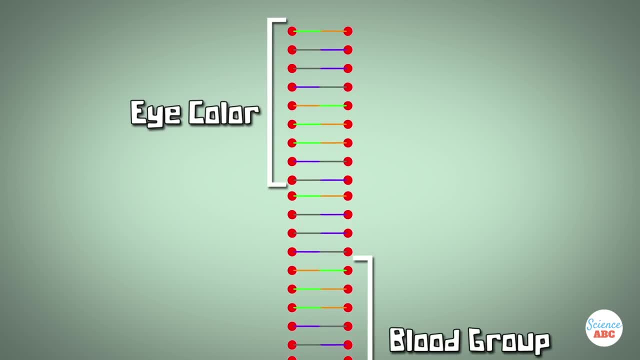 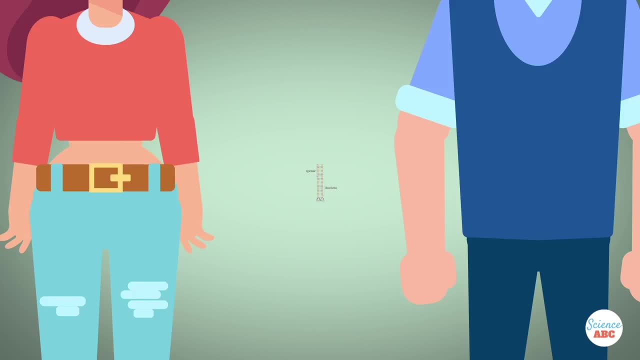 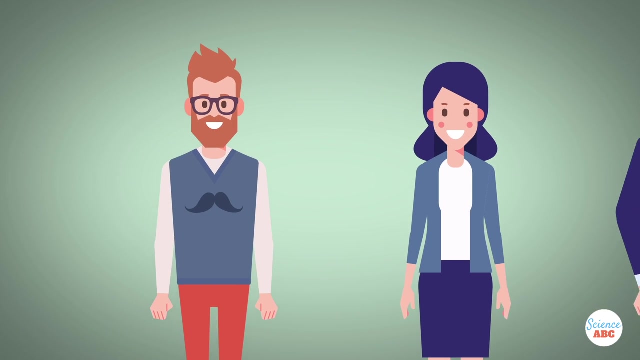 like eye color or blood group, Genes can come in a variety of flavors, meaning that the gene for eye color can code for blue eyes or brown eyes, or even green eyes. Each of us possess a unique combination of these genes, giving some of us brown eyes with blonde hair or blue eyes with brown hair. 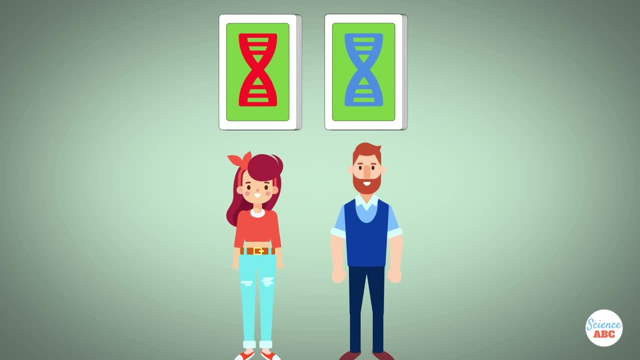 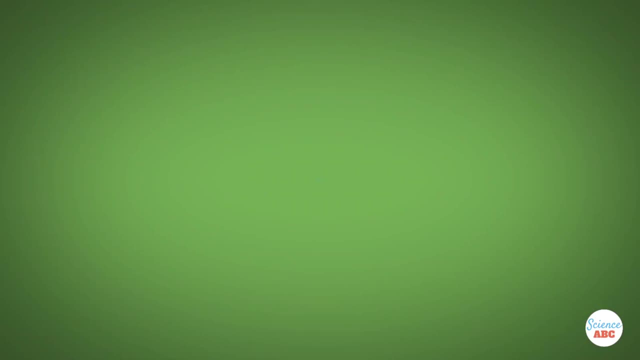 Now these different flavors of genes get all mixed and rematched in a process called recombination, which happens when organisms mate. In the nucleus of a cell, long twisted ladder-like strands of DNA are formed into compact chromosomes. Chromosomes come in pairs. Humans, for example, have 23 pairs of chromosomes, one from the mother and one from the father. 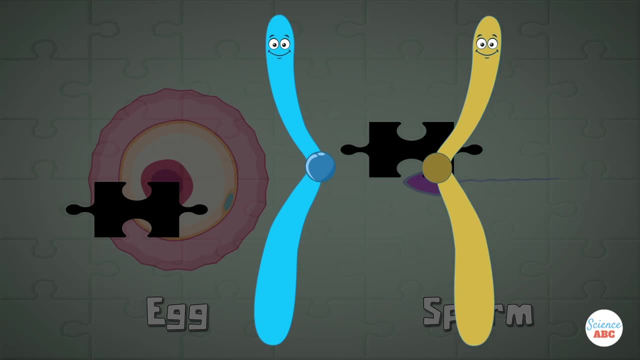 In the process of creating the egg and the sperm, the chromosomes pair up and then swap parts of their DNA. This is recombination. Once this recombination happens, the paired-up chromosomes are then separated and the resulting eggs and sperm have only one half of the chromosome pair. 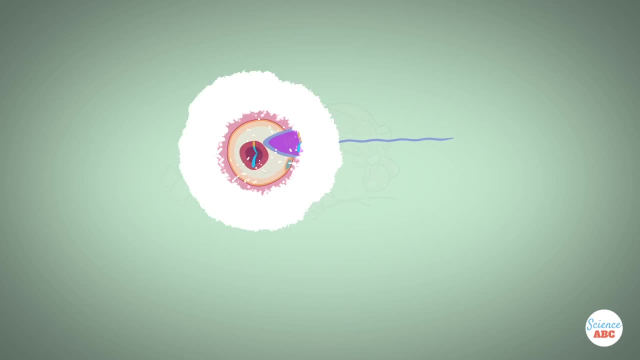 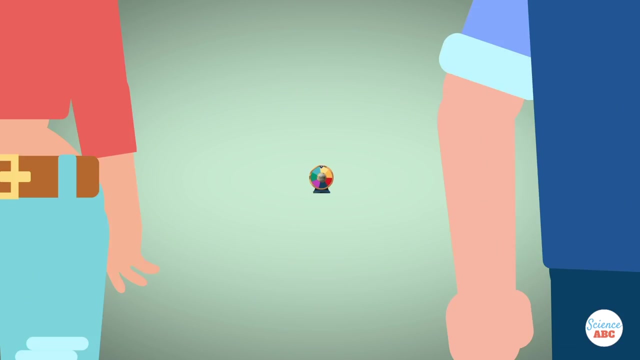 Then, when two people mate, a random egg and a random sperm will fuse together to create new life. Recombination creates combinations of genes that are unique to each one of us, thus creating new life. This is why you and your siblings don't look identical. 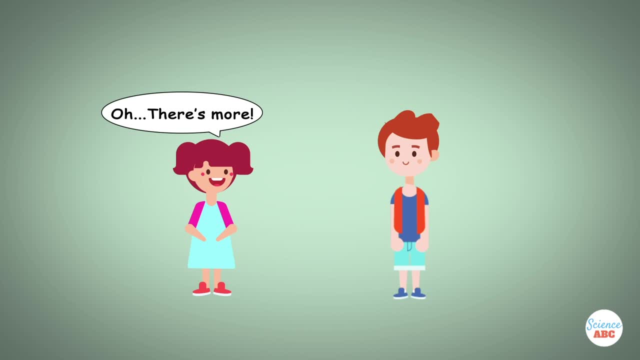 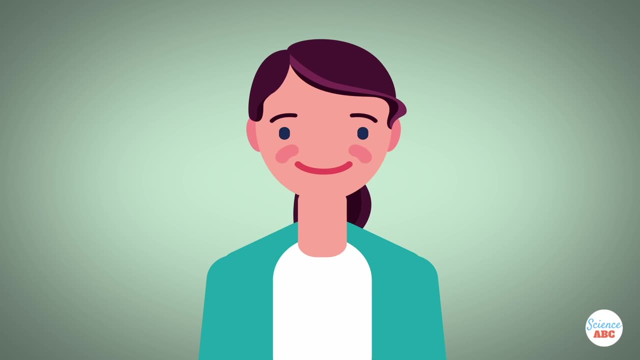 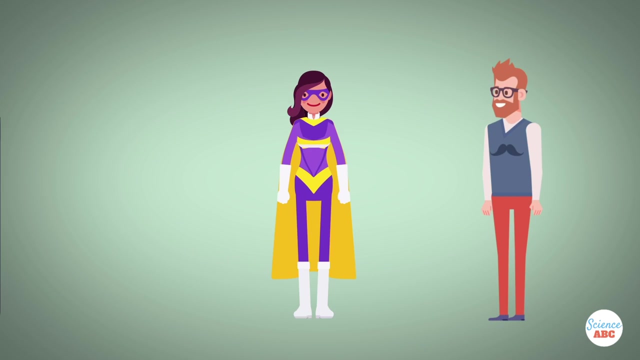 Recombination isn't the only way that variety develops. Another process is mutation, which is a change in the DNA sequence. Mutations can either modify traits like a new eye color, or create a completely new trait. The sad news is that most mutations won't make you Jean Grey or Wolverine. In fact, most mutations don't cause any change at all. They are effectively neutral. Some of them can even cause a nepotism, but in a few cases mutations can be good, like a mutation that allows animals to camouflage and hide from predators. 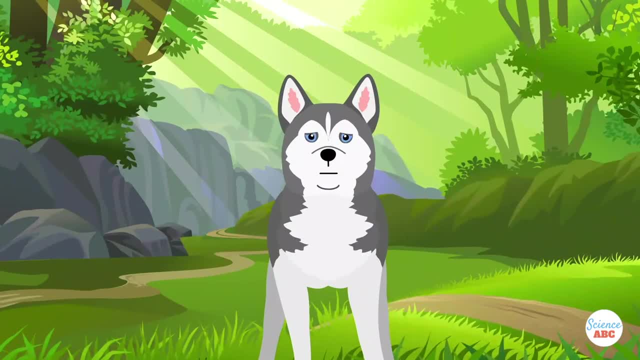 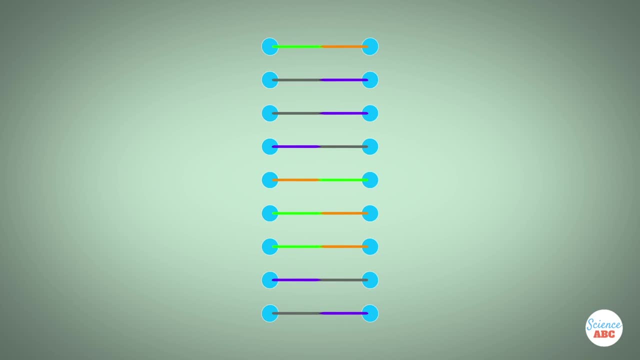 or produce a scent that makes it extremely appealing to the opposite sex, whereas bad mutations are those that cause diseases or weaken an organism. Mutations can occur randomly, or it can happen when DNA divides and the cell's machines make mistakes, Or it could even happen from external factors such as radiation or when viruses infect us. 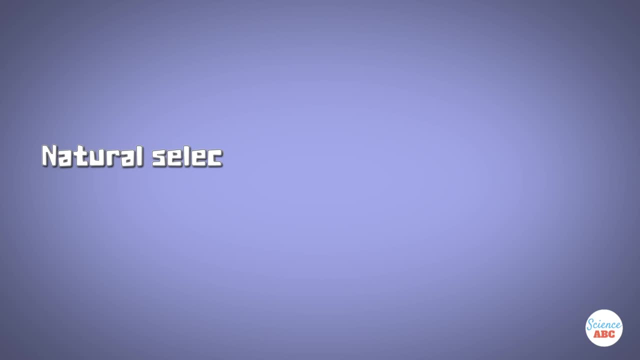 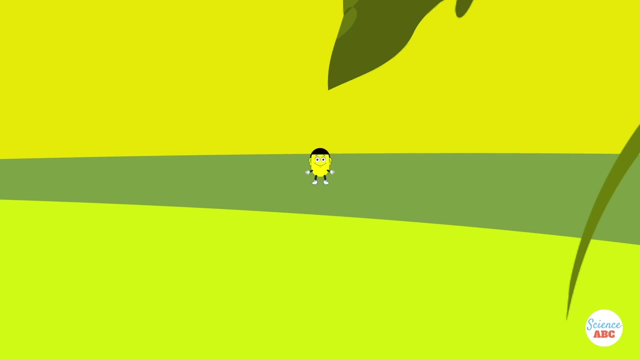 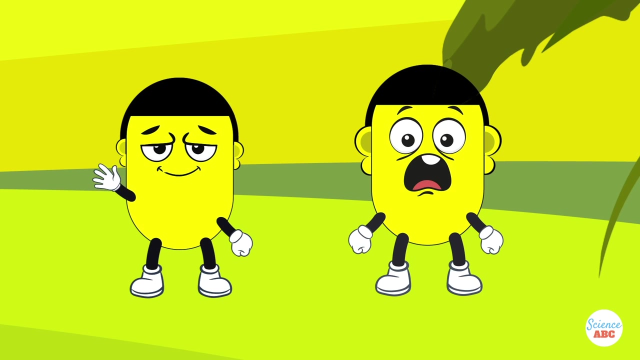 selection and genetic drift. Natural selection is a process where the environment selects traits that allow the individual or group to survive best. Consider a hypothetical organism that gets a mutation one day that gives it heightened hearing. This better hearing allows it to detect and flee from predators faster so that it lives longer. It passes this better hearing to its 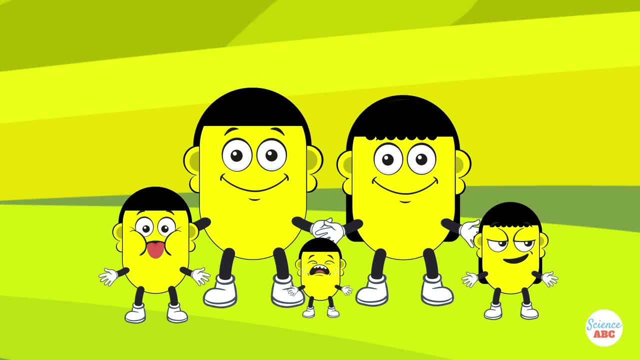 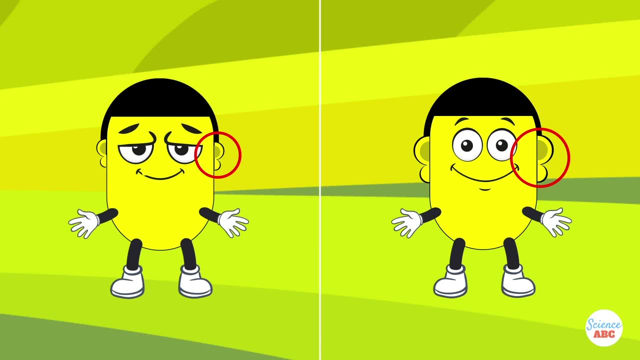 offspring, who also survive longer than organisms that don't hear as well. Soon, there are many better-hearing individuals in the group This better hearing was selected for. On the other hand, if an individual can't hear as well, it is less likely to survive. 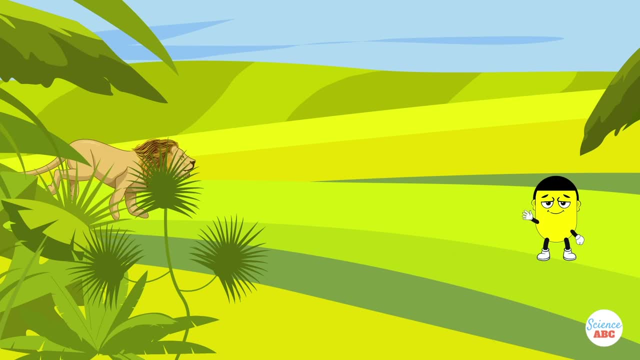 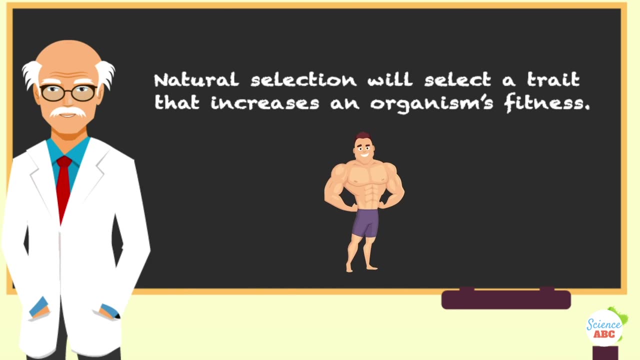 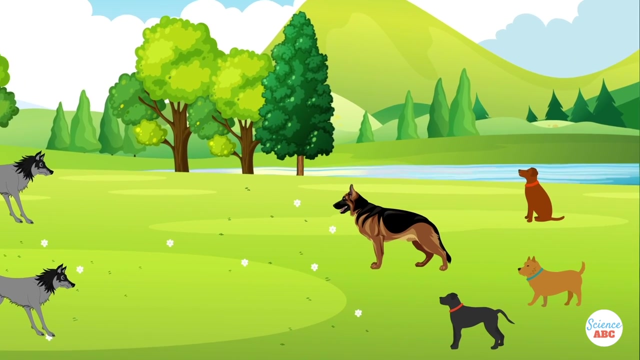 long enough to reproduce and pass those genes on to its offspring. Natural selection will select a trait that increases an organism's fitness. Here, fitness doesn't mean strength. It means anything that will aid the animal in survival and reproduction. The modern dog evolved from wolves. However, instead of the environment doing the selecting, 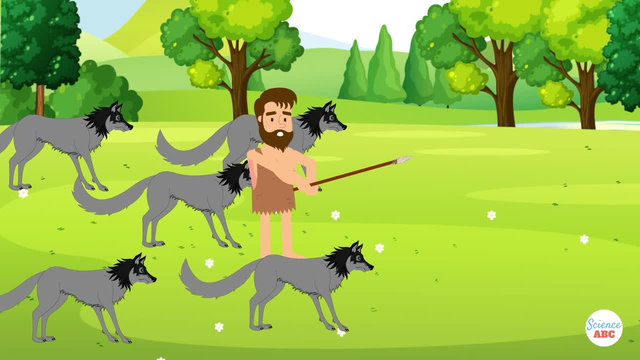 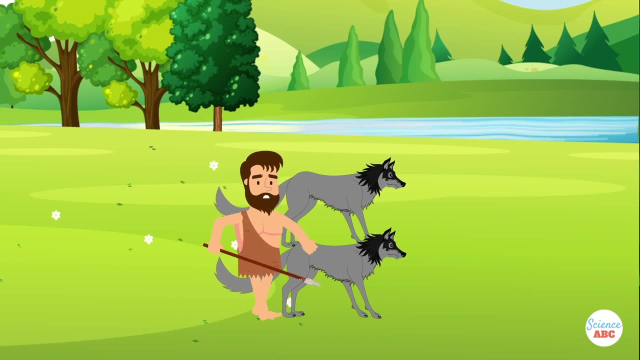 it was humans. Humans selected those traits in wolves that made them better companions, including loyalty and a more docile temperament. The wolves that showed these traits were bred Over time. humans selected and mixed these traits, resulting in the wide variety of dog breeds we 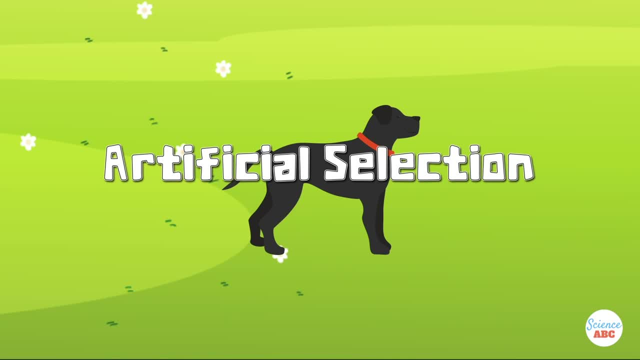 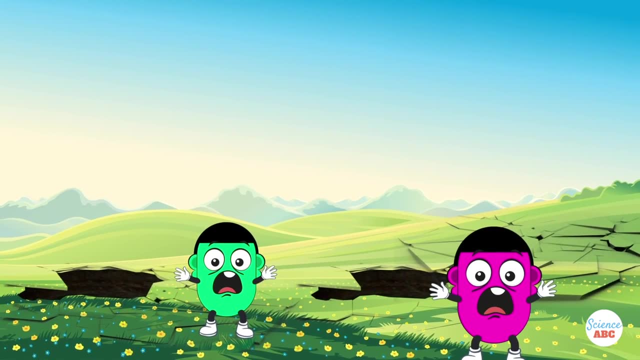 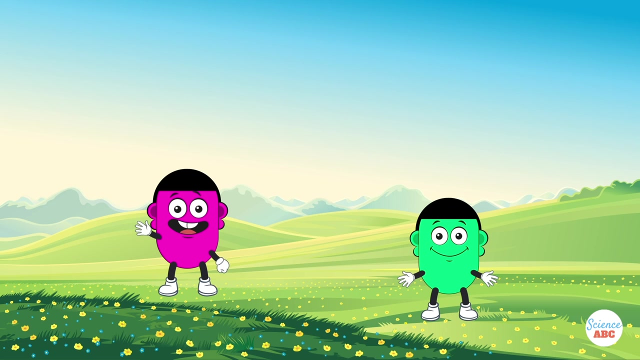 see today, This is called artificial selection. Sometimes, though, luck also plays a role in how animals evolve. For example, a natural catastrophe can destroy the majority of a given population. The individuals that remain are there by mere chance, so the traits that remain in the gene pool aren't. 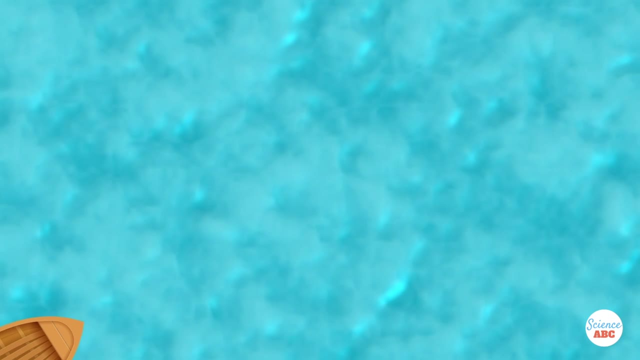 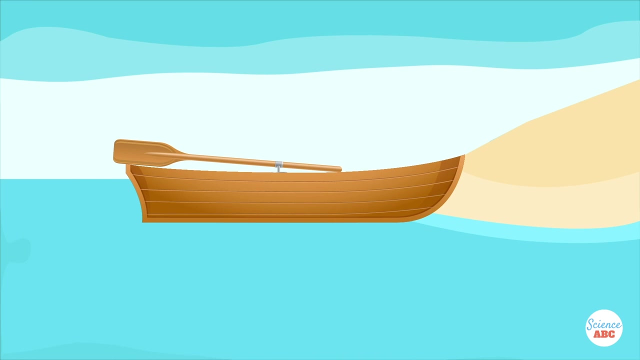 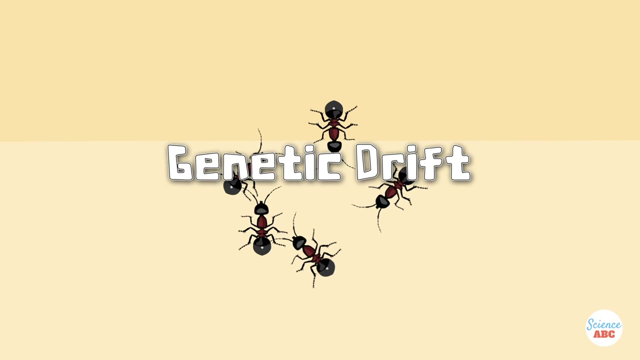 necessarily any better suited for their environment. Or perhaps an organism or population somehow finds itself in a completely new place, separated from its normal reproductive population. The individuals in this new place will now evolve and spread in that area. This is called genetic drift. Though natural selection chooses traits that enable survival, it isn't perfect. Diseases and certain disorders aren't necessarily eliminated, even though they cause pain. Furthermore, traits that no longer serve a purpose will not be actively selected against unless they become detrimental for survival. They will similarly be passed down to future. 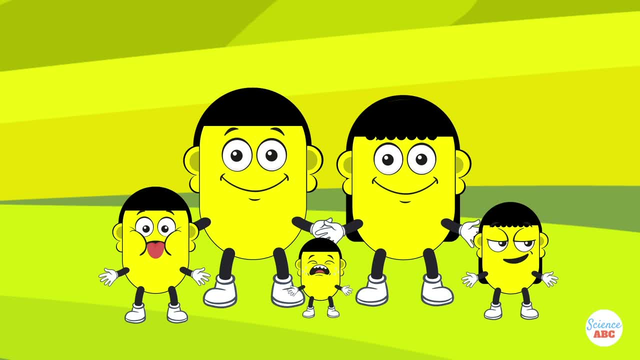 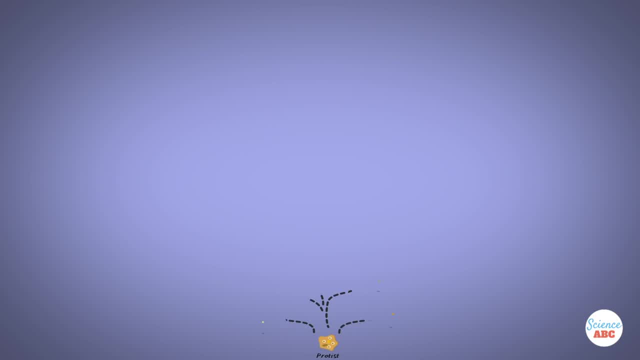 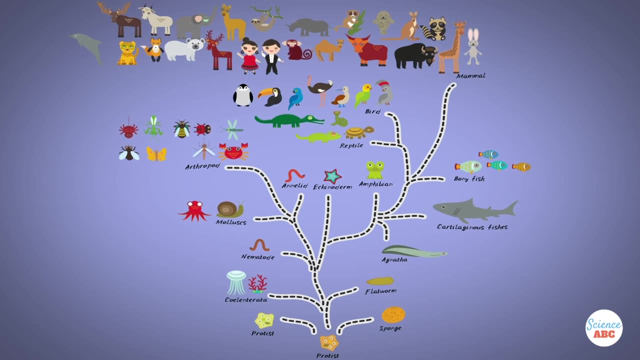 generations, if the animal manages to live long enough to mate Speciation. Thus far, we've only spoken about evolution within a single group, But life is a tree with thousands of branches to different species. And how do these species evolve? This occurs through a long process of speciation. 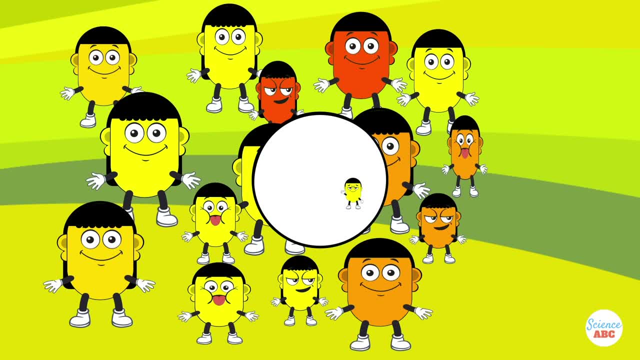 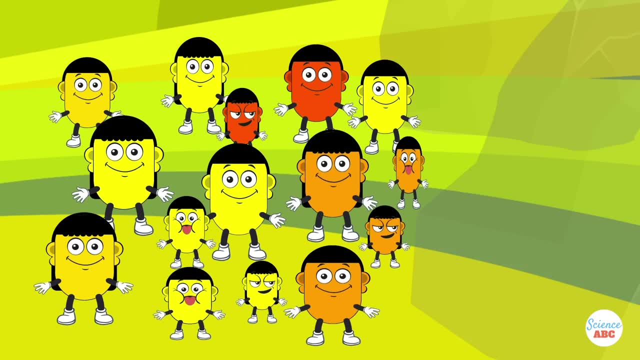 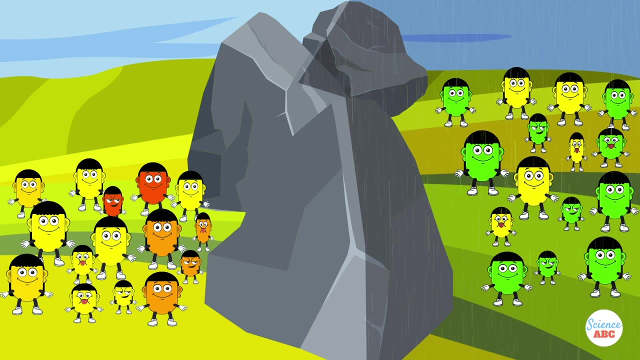 Over time, mutations, recombination events, natural selection, luck and other factors create a gulf of differences within a population that was once homogenous. These changes might happen because of a literal geographic barrier that separates a population. The environments on either side of the barrier might be different and over many years they might be different and over 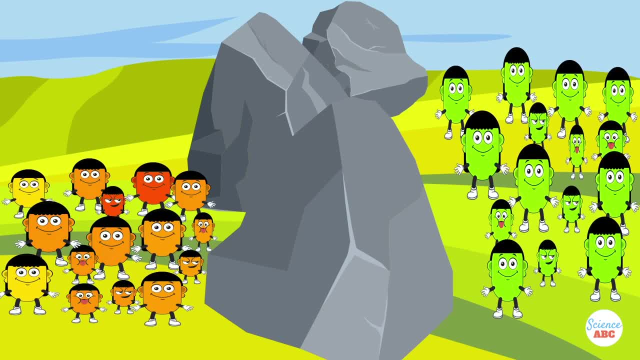 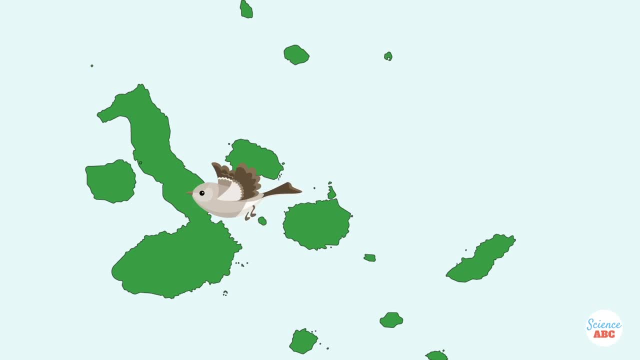 many generations, the two populations become different species. This happened with Darwin's finches on the Galapagos Islands. At one point, the finches' ancestors from the mainland must have migrated to the islands. The islands were rich in food resources and each had a slightly different food profile. 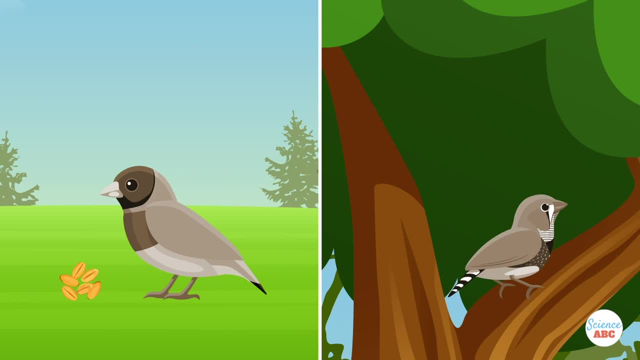 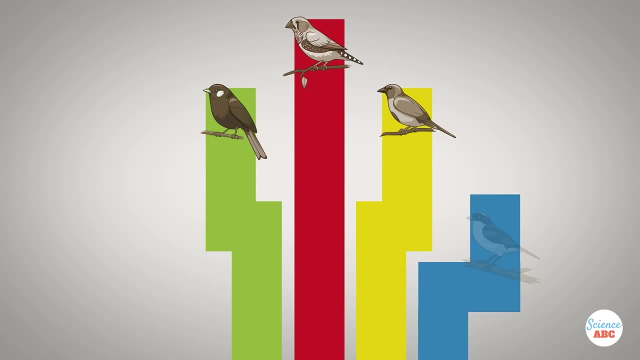 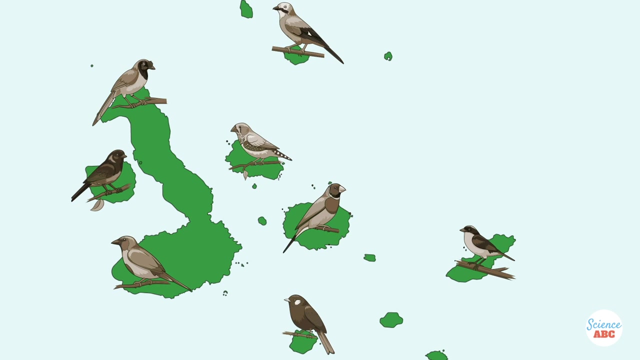 Due to this variation, the birds with longer beaks could survive on insects, whereas those with blunter beaks fed on seeds and leaves. Over many generations, evolution took over and distinctly different finch species evolved. Once a new species comes into being, it doesn't necessarily mean that the old species vanishes. 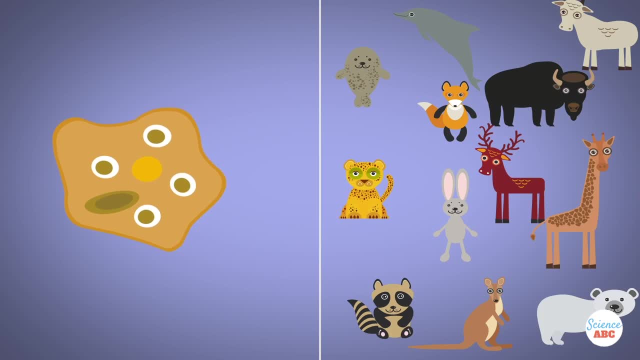 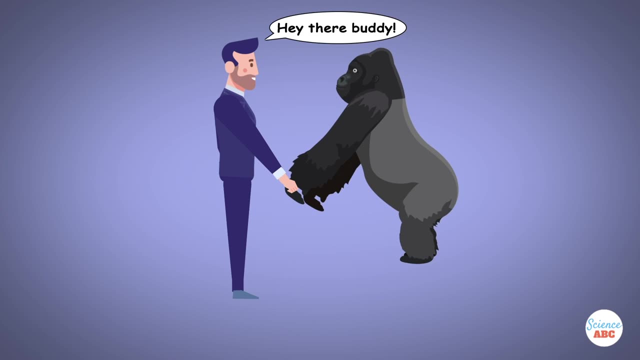 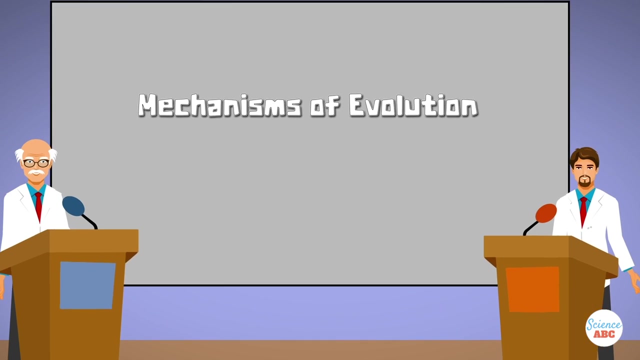 Just as single-celled bacteria didn't go extinct just because multicellular life evolved, similarly old life does not simply go extinct because a new species appears on the scene. Each can tap a different resource and exist in their new habitats. The evolution of life doesn't only act through one mechanism. The main debate revolves around 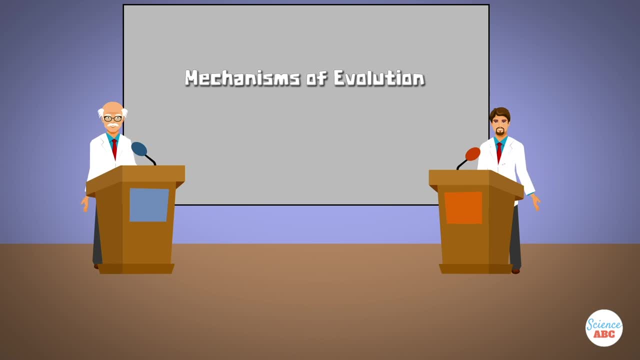 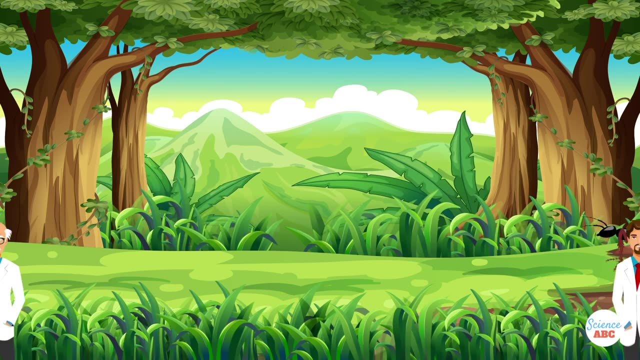 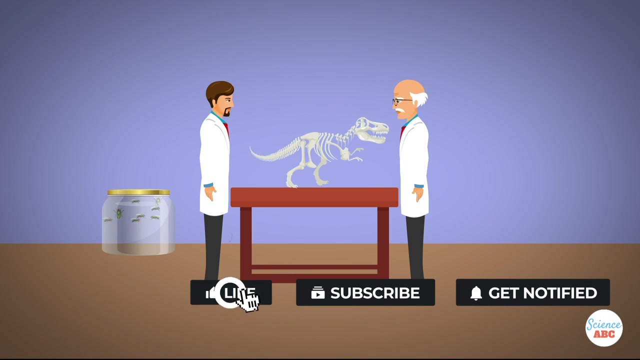 how much one mechanism contributed to the changes we see today. Do deer have antlers because they want to look sexy, or is it simply a byproduct of some other change? Did insects get smaller because of a lack of oxygen or predators, or both? Scientists study evolution in the lab and 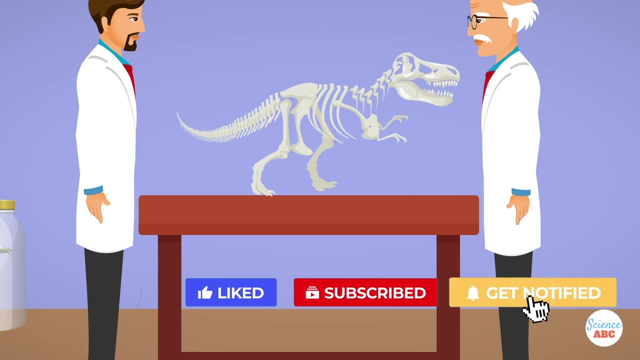 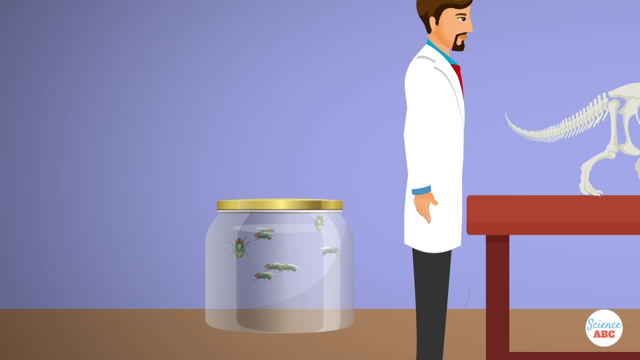 through the fossil record. We know how whales evolved through the existence of intermediate fossils. In the lab, we breed bacteria, flies and worms to see how they evolve under different conditions. We know how whales evolve through the existence of intermediate fossils. In the lab, we breed bacteria, flies and worms to see how they evolve under different conditions. 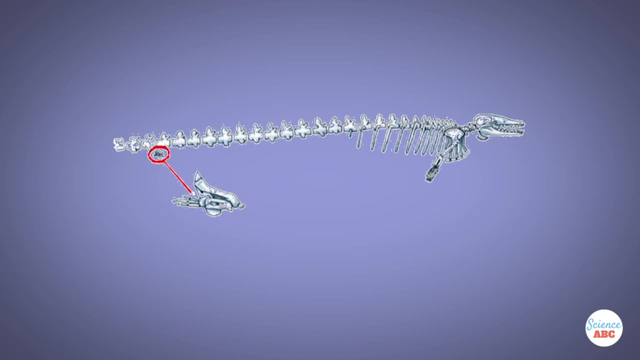 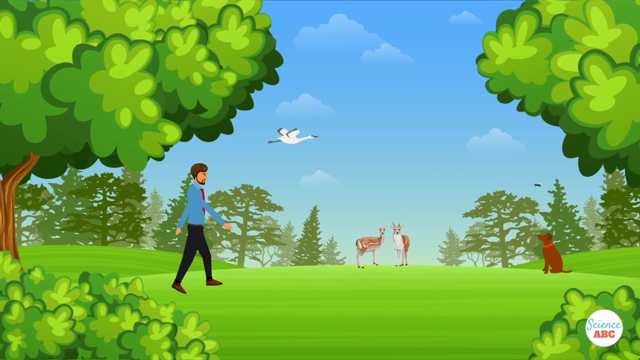 This evidence gives us some hint at how life reached such an astonishing level of diversity. With all that in mind, take a moment to notice the diversity on our incredible planet and appreciate that it took four billion years of evolution to lead not only to you.